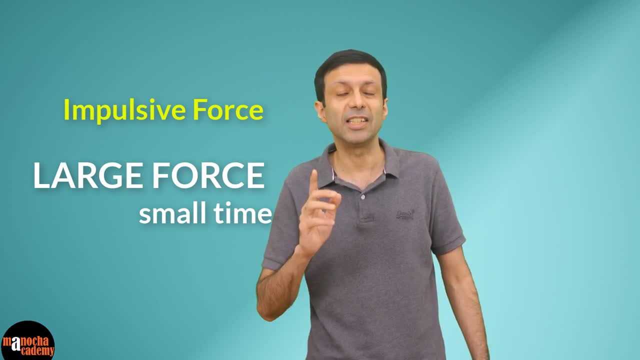 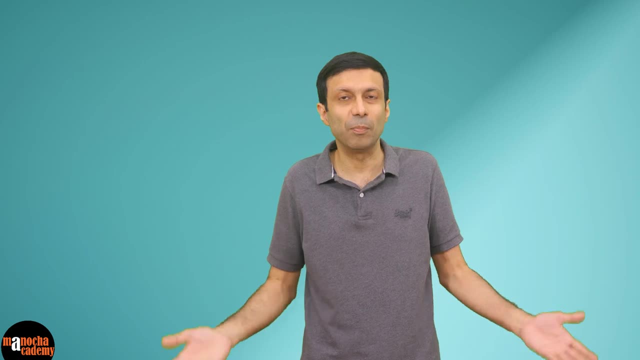 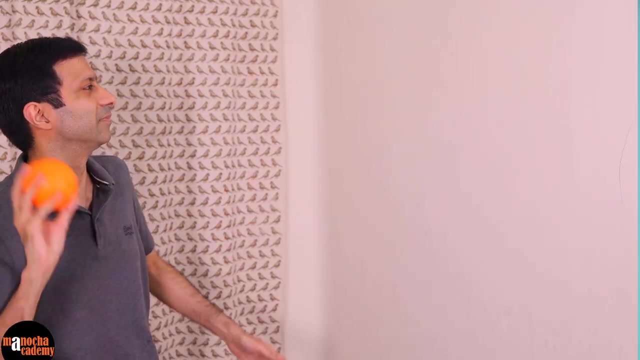 an impulsive force. In physics, the concept of impulse is used when there is a large force that acts for a small duration. We can understand the impulse in the simple way by using the ball bouncing example. When the ball hits the wall, it rebounds back. When the wall has just bounced back, it отделans. 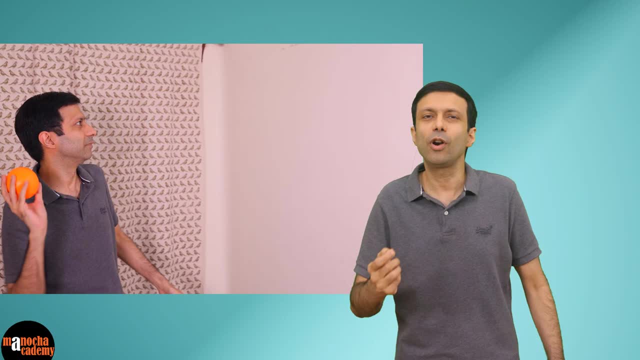 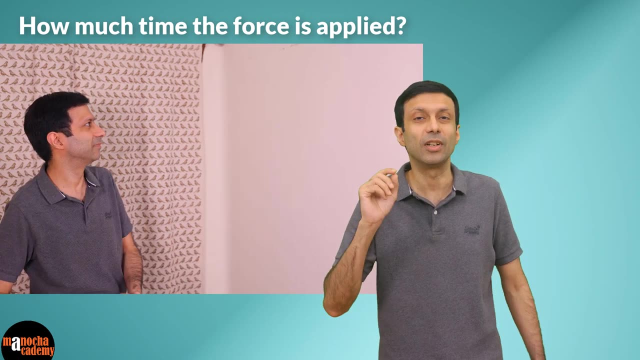 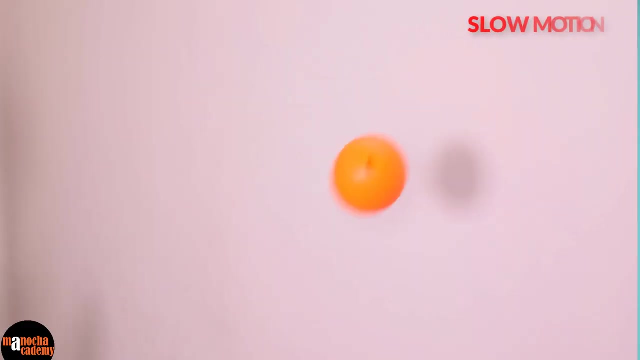 ball and it reverses the motion of the ball. For how much time does the wall apply the force on the ball? The ball bounces back really fast, so the time that the force is applied is really small. Even if you watch the video in slow motion, can you see, it is very hard to determine the 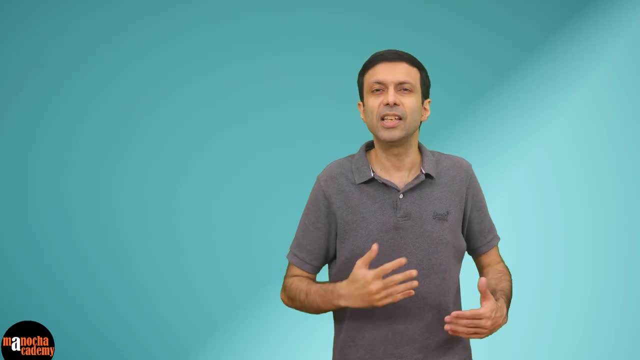 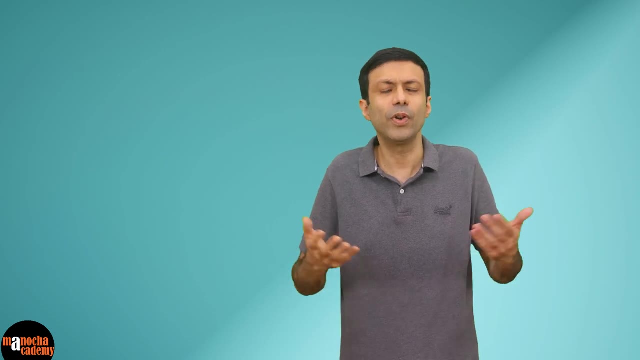 time when the ball is in contact with the wall. Since the force acts for such a small time, it is very difficult to measure the force accurately. So what do we do here? Force and time duration of the force are both difficult to measure. 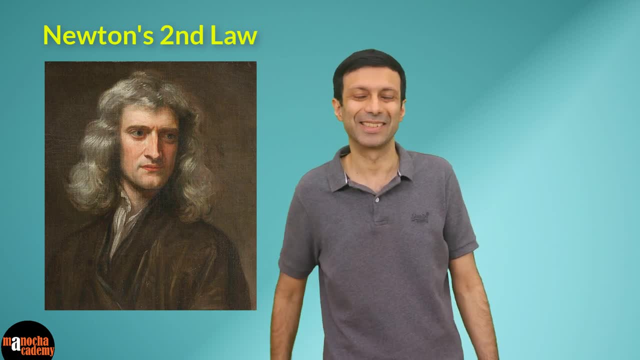 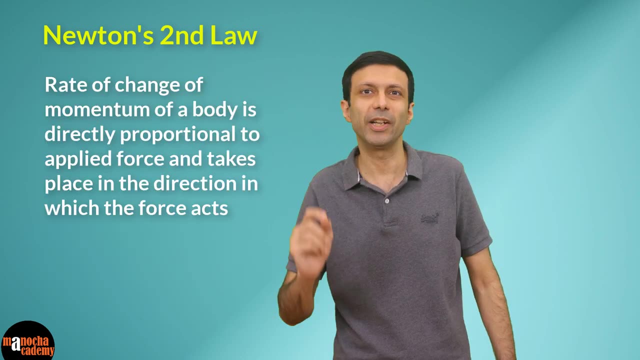 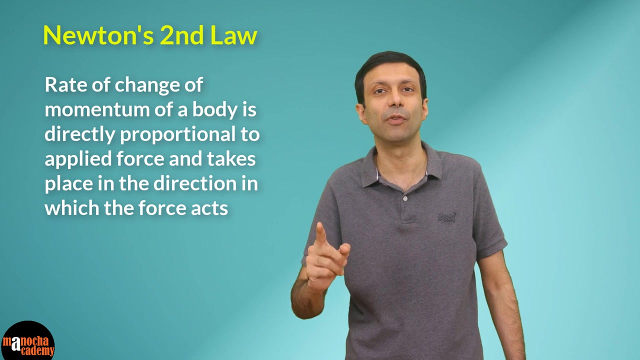 Let's see if Newton's second law of motion can help us here. Do you remember Newton's second law? Newton's second law of motion states that rate of change of momentum of a body is directly proportional to the applied force and takes place in the direction in which the force 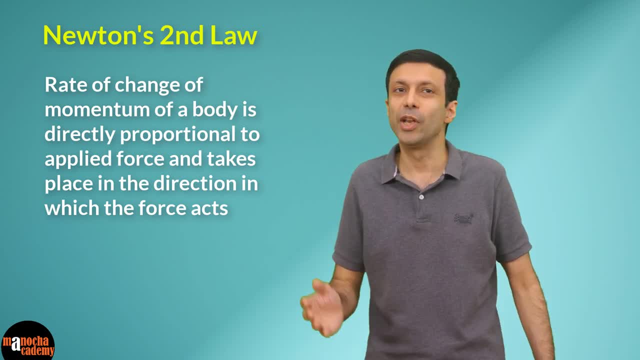 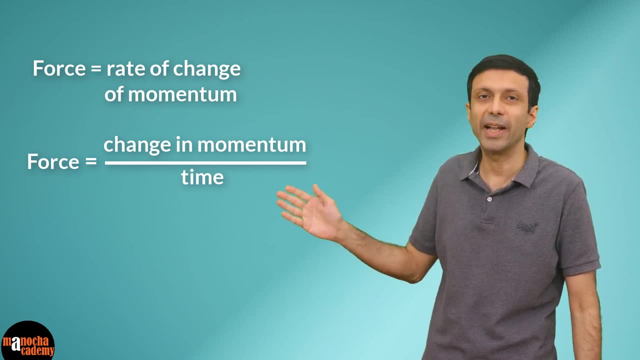 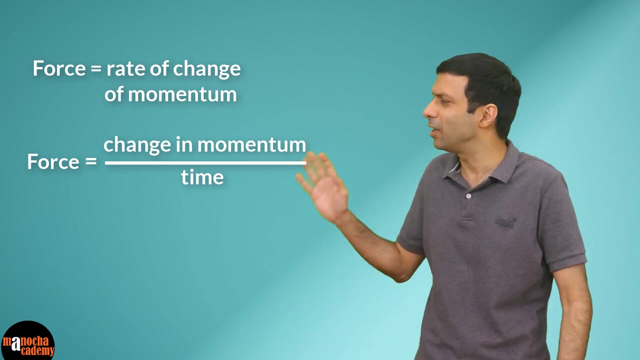 acts. From Newton's second law of motion, We know that force equals rate of change of momentum, That is, change of momentum divided by the time. Now, since force and time are difficult to measure here, let's keep both these difficult guys on one side. 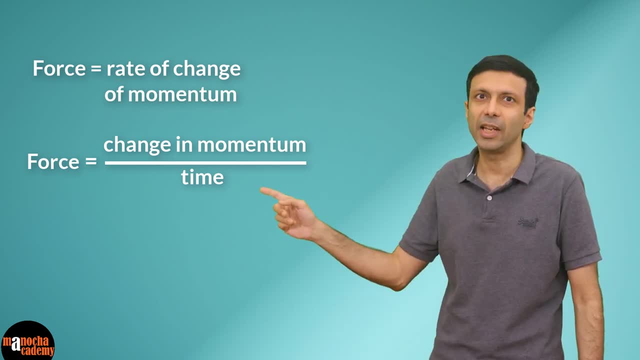 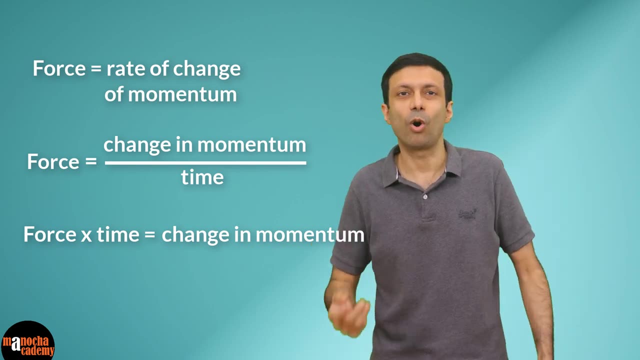 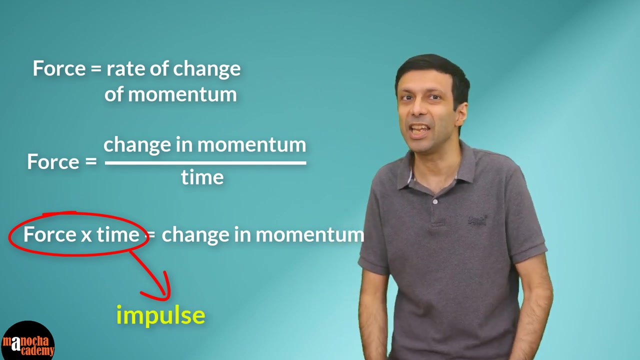 So I am going to take time to the left hand side and we get the equation as: force multiplied by time equals change in momentum. This product of force multiplied by time equals change in momentum. The force multiplied by time duration is defined as impulse. So impulse equals to the change in momentum of the body. 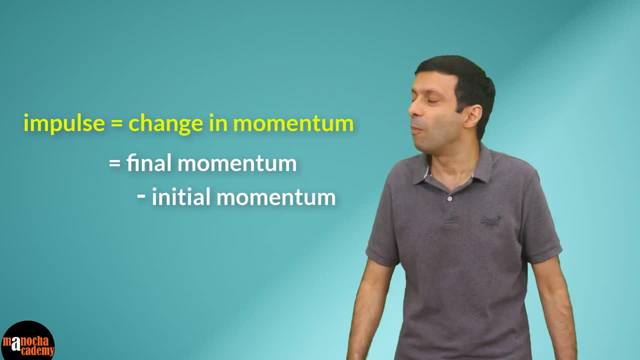 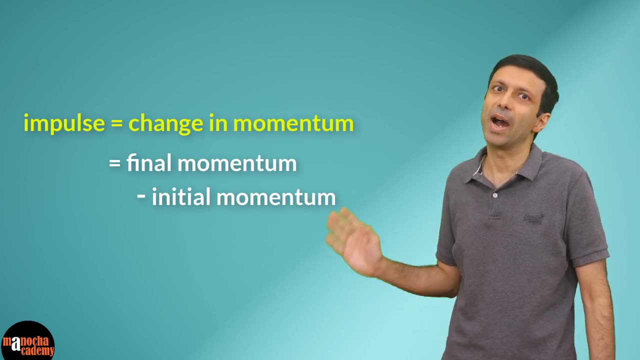 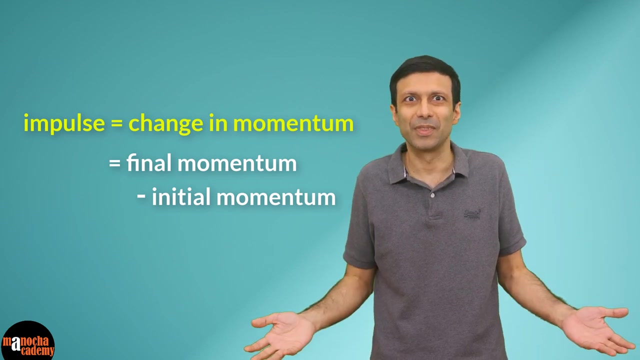 Change in momentum can be calculated as final momentum minus the initial momentum. So remember, it is never initial minus final, It is always final momentum minus the initial momentum. So impulse, which is the change in momentum, can now be easily measured. So the trick is: 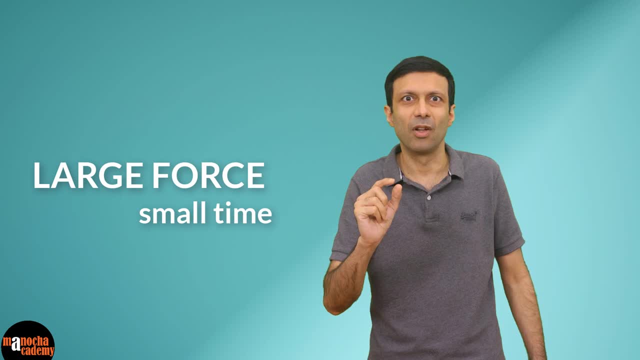 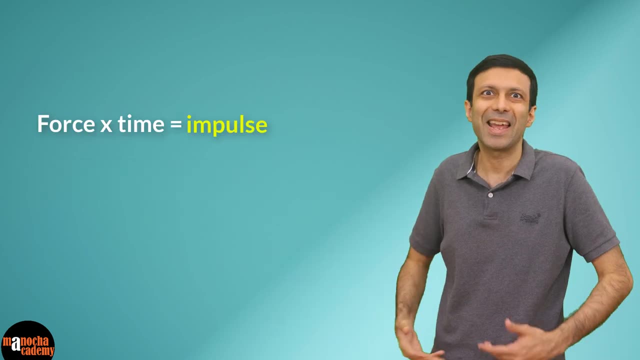 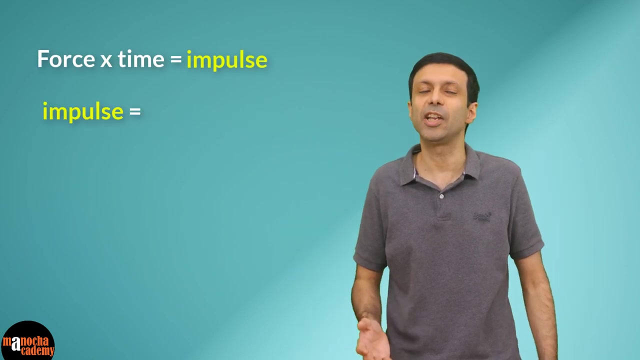 That when you have a large force for a short time. Force and time are difficult to measure. But the product, that is, force multiplied by time, can be measured easily and it is called the impulse. Impulse is a measurable quantity and is equal to the change in momentum of the body. 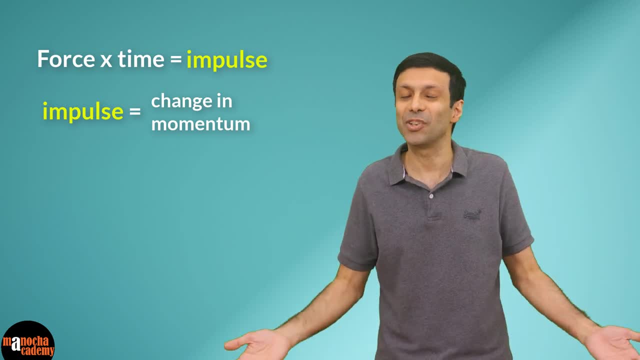 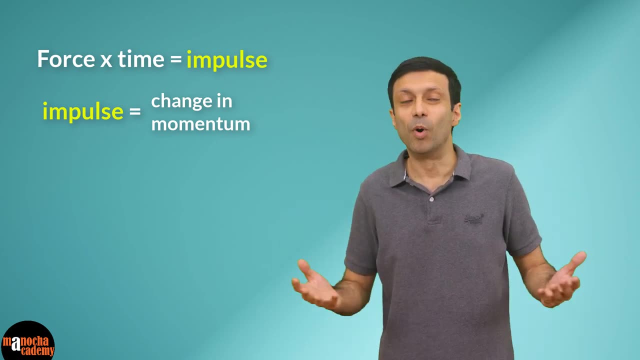 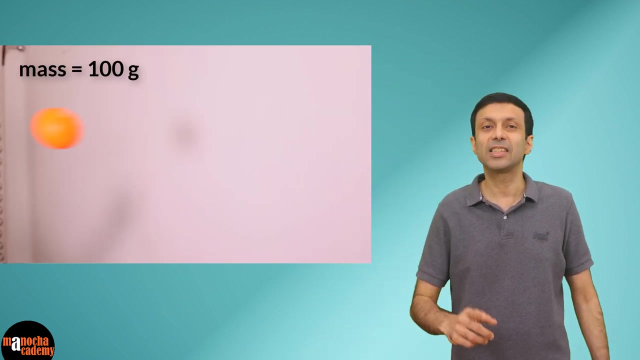 So let's see if we can calculate the impulse of the ball when we hit it on the wall. We will use the formula: Impulse equals change in momentum. Remember momentum is the product of mass and velocity. Let's say the mass of the ball is 100 grams. 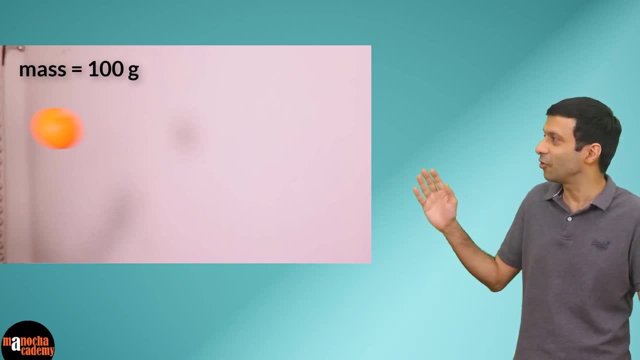 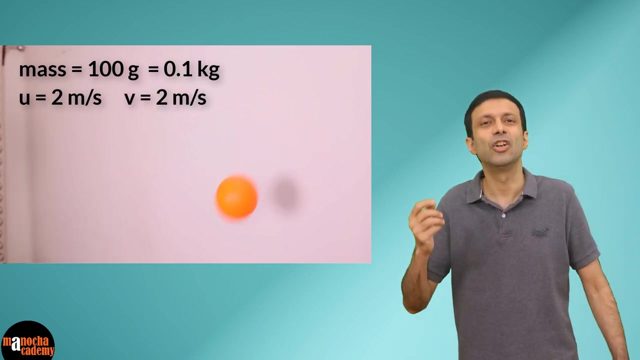 Let's convert the mass into SI unit. So mass: 100 grams equals 0.1 kilogram. Let's say the velocity with which the ball hits the wall is 2 meters per second. The ball rebounds with the same velocity, So the return velocity is again 2 meters per second. 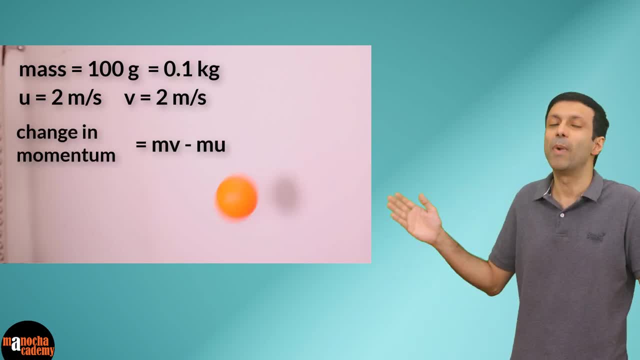 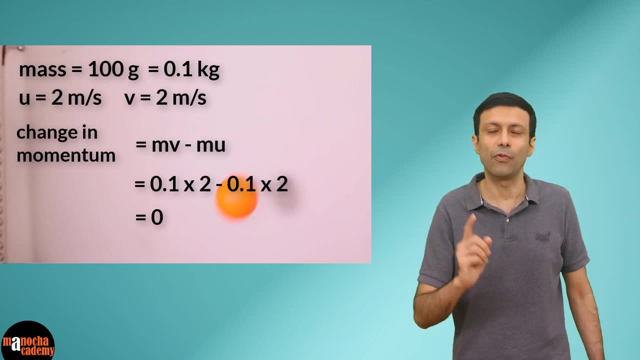 So the change in momentum here is 2 meters per second. The momentum here is going to be the final momentum minus the initial momentum, That is, mv minus mu. So if you plug in these values into the formula, you will get an answer of zero. 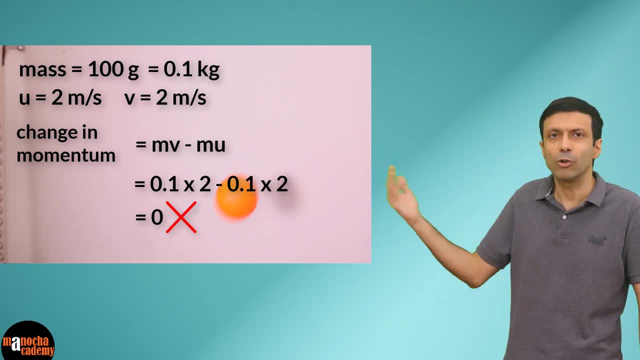 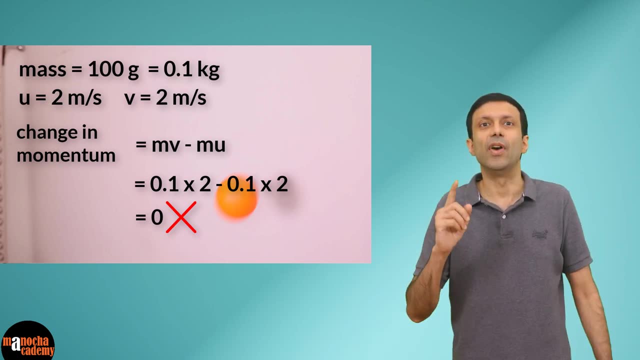 But the change of momentum can't be zero, since the ball is bouncing back, The wall is applying a force on the ball. So what went wrong here? Remember, velocity is a vector quantity. It has both magnitude and direction. So after collision with the wall, the ball moves in the opposite direction. 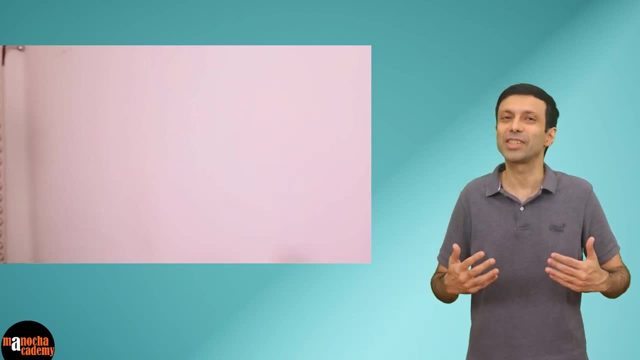 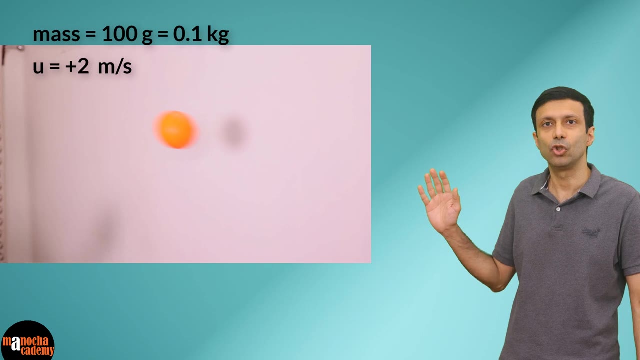 So we need to take one velocity as positive and the other velocity as negative. Here I am going to take the initial velocity as positive, So the initial velocity is 2 meters per second and the final velocity, which is after the collision with the wall, is negative. 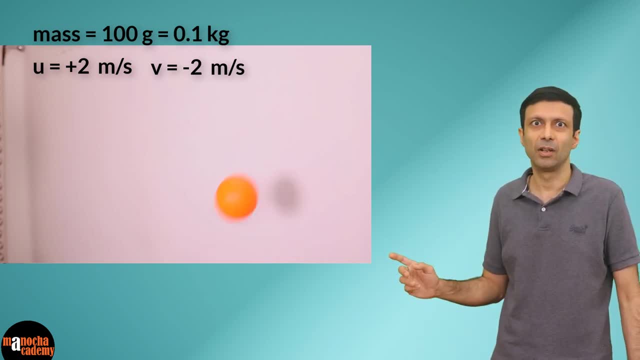 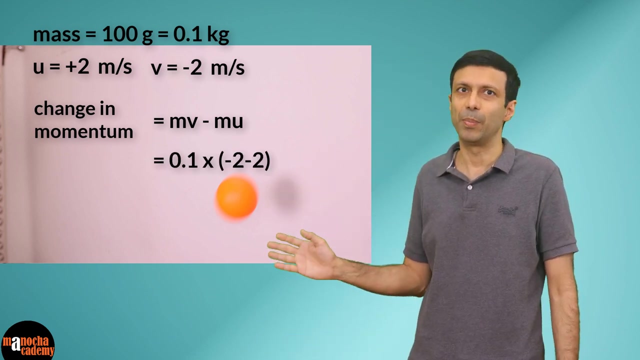 So it will be minus 2 meters per second. So you can also take the reverse as well, But this is what I have taken here, The initial velocity as positive and the final velocity as negative. Now let's plug in these correct values into our formula and calculate the impulse. 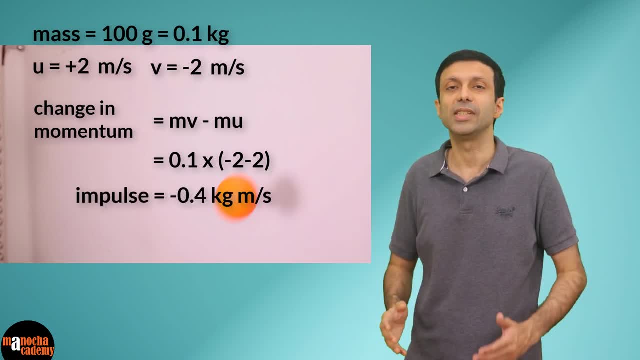 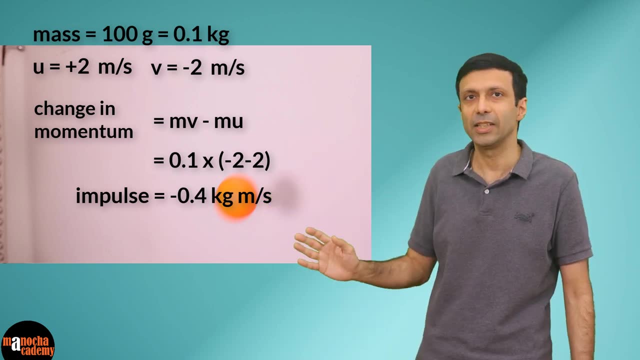 The impulse is going to be the change in momentum, which is mv minus mu, So that's going to be 0.1 multiplied by minus 2, minus 2.. So we are getting the answer as minus 0.4 kg meter per second. 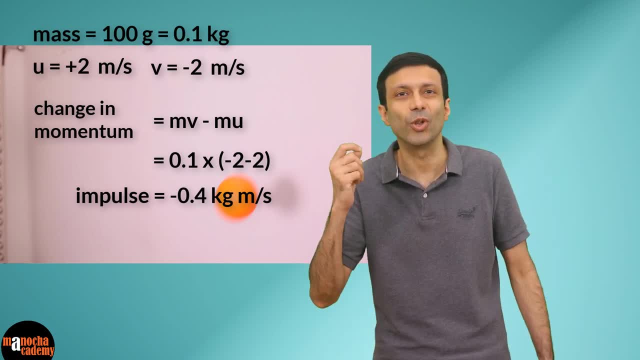 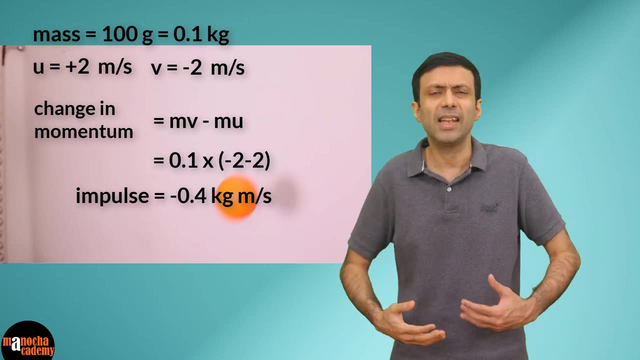 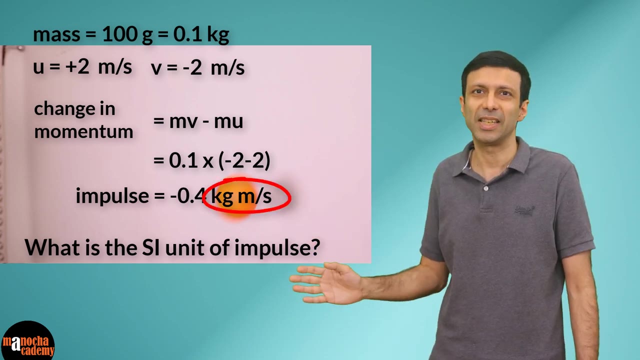 This is the impulse that the ball is bouncing back. The ball applies on the ball. It is the product of force multiplied by the time duration. Now what is the SI unit of impulse? As you can see from our calculations, we got the unit as kg meter per second. 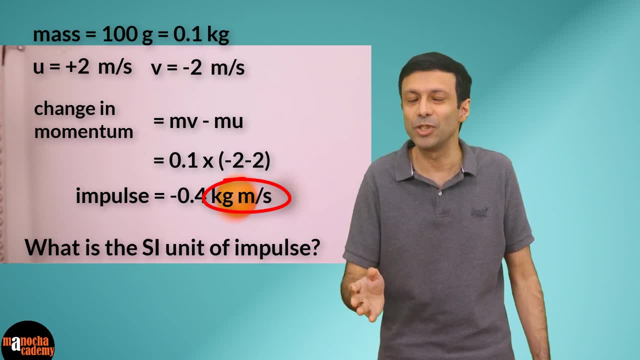 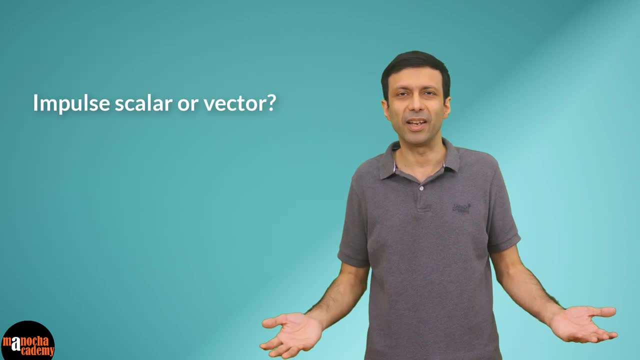 It has the same unit as momentum, as impulse equals to the change in momentum. Now, is impulse a scalar quantity or a vector quantity? What do you think That's right? It is a vector quantity, Since momentum, or change in momentum, is also a vector. 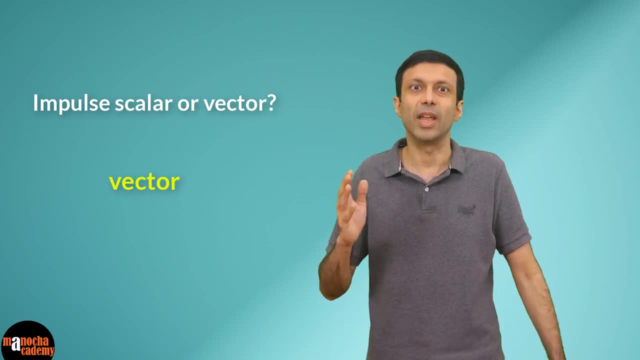 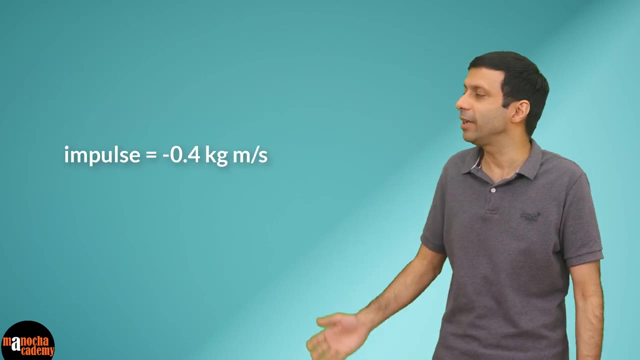 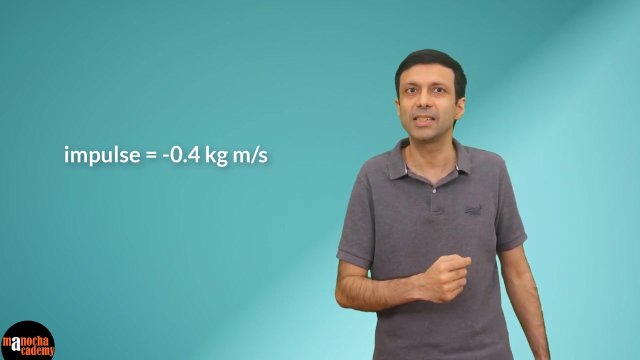 It has the same direction as the velocity, which is a vector. So impulse is also a vector quantity. It has both magnitude and direction. Here we calculated the impulse as minus 0.4 kg meter per second. So the magnitude or the value of the impulse is 0.4 kg meter per second and it has a negative. 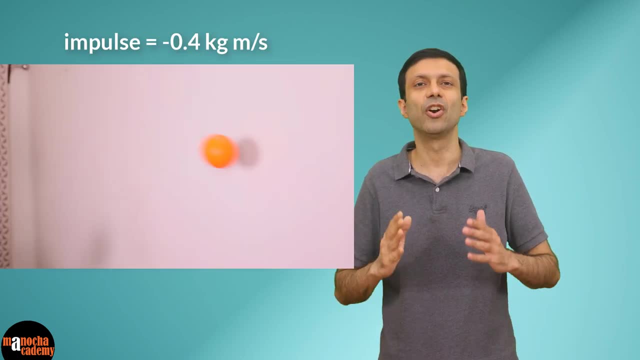 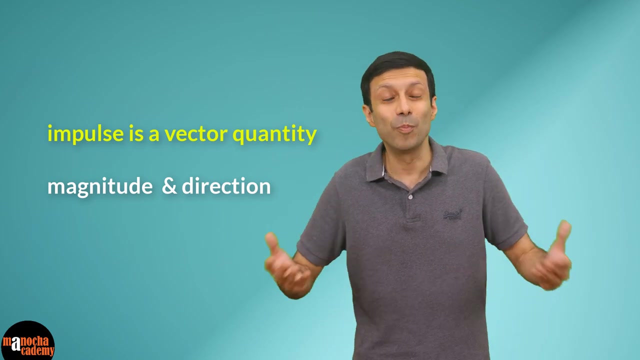 sign, Since the force is in the opposite direction. So the force makes the ball go back from the wall. So remember, impulse is a vector quantity. It has both a magnitude and a direction. Now a football quiz question for you. Do you know who holds the record for the fastest football kick? 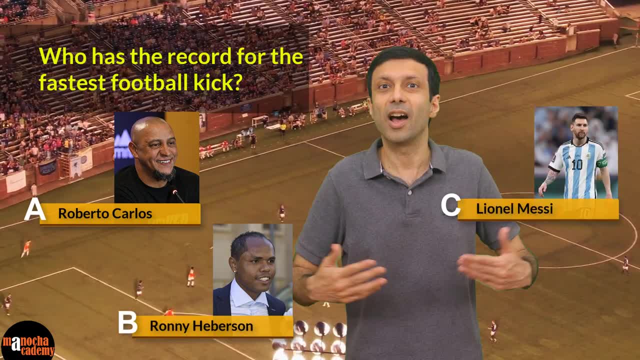 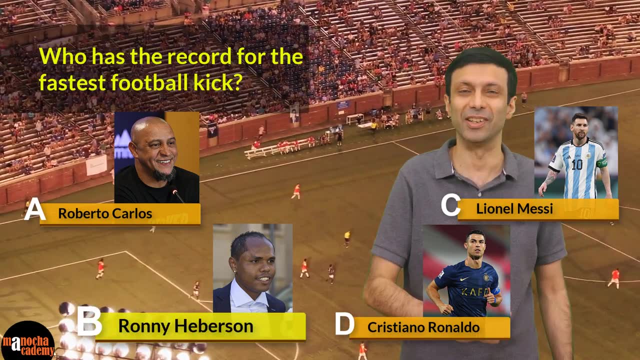 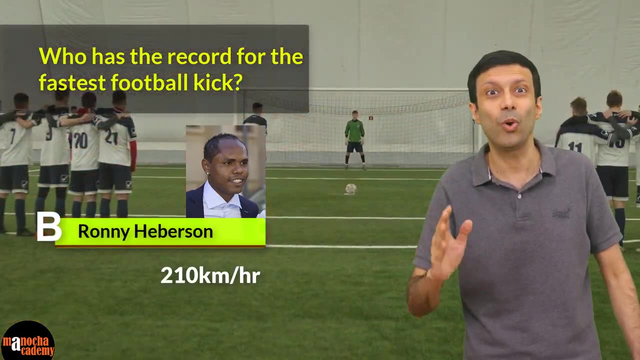 Is it Roboto Carlos? Ronnie Heberson, Lionel Messi or Cristiano Ronaldo? What do you think? The correct answer is Ronnie Heberson, the Brazilian footballer. Believe it or not, he kicked the ball at an amazing speed of 210 km per hour. 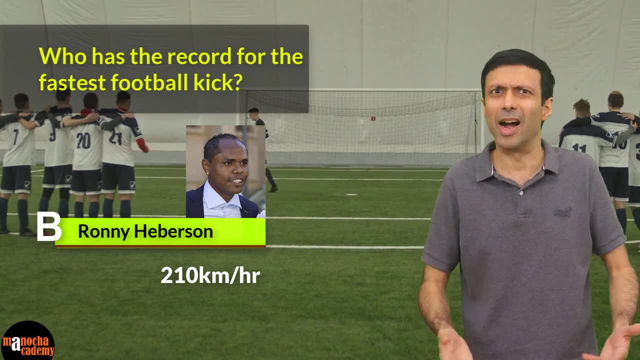 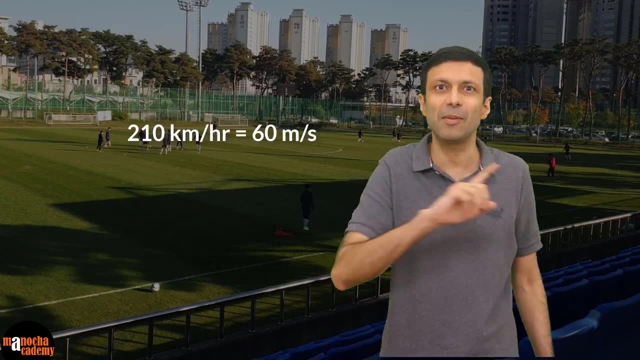 And no guesses. of course he scored a goal. I don't think the goalkeeper or anybody saw that ball. 210 km per hour is about 60 meters per second. The mass of the football is about 400 grams. So based on these numbers,